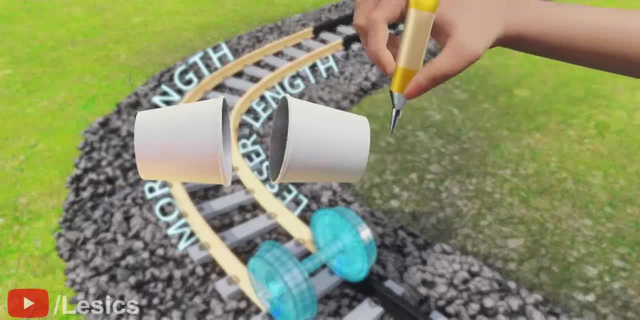 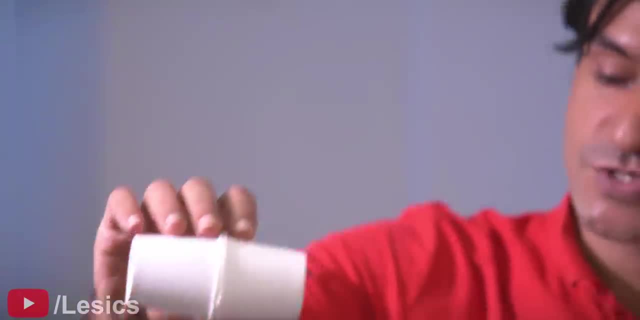 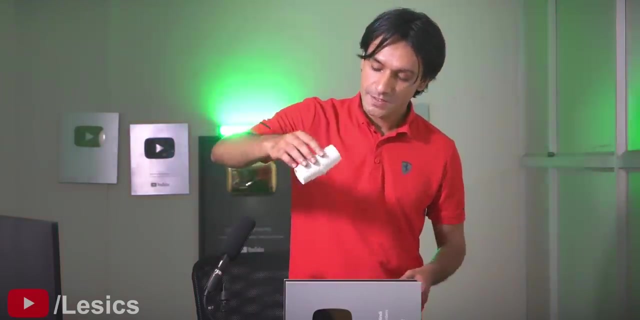 To understand the first accomplishment, let's consider a simple experiment with glued paper cups. When I roll this set of glued paper cups on these tracks, you can see that they are moving perfectly straight, Even if I try to give a small tilt for the cups at the beginning. 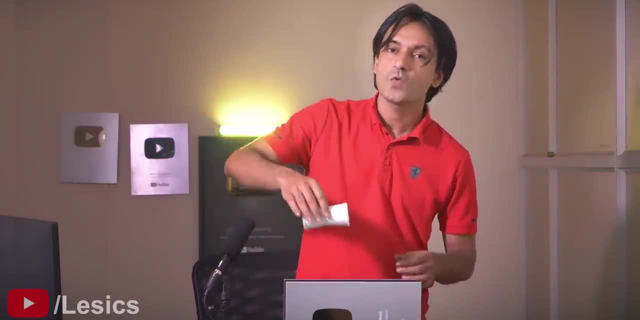 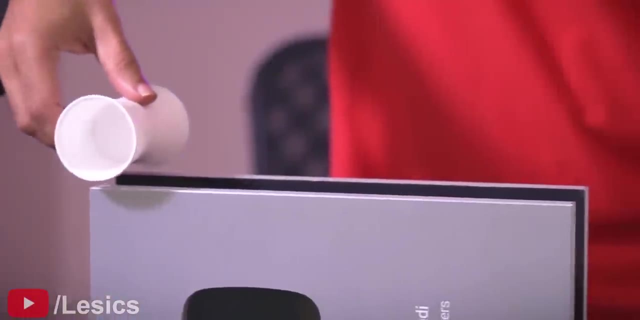 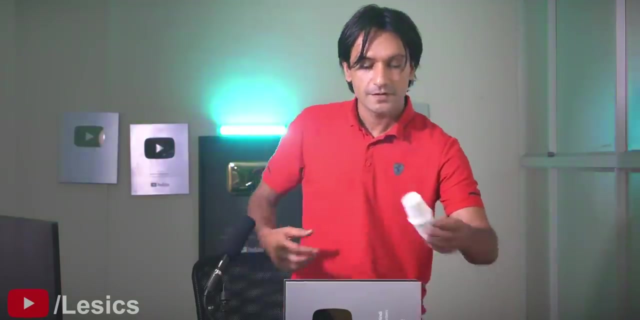 they are still managing. Now, what about this set? This is glued in opposite way. When I roll the cups on the same track, it is failing. The wheels in this set are not perfectly conical. Railway wheels use this kind of conical shape. This angle makes 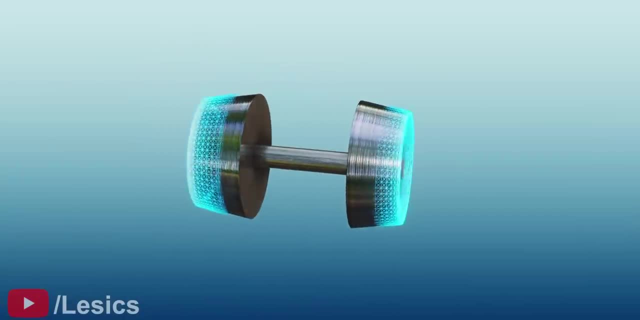 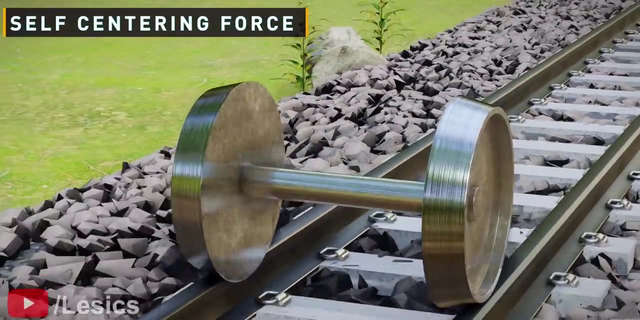 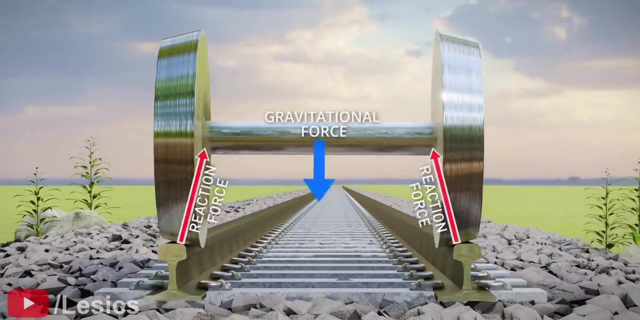 sure that the wheels will never leave the track, But the question is why This conical arrangement produces a self-centering force. To understand how we need to check out the forces acting on the wheels During a straight track movement, the main forces acting on the wheels. 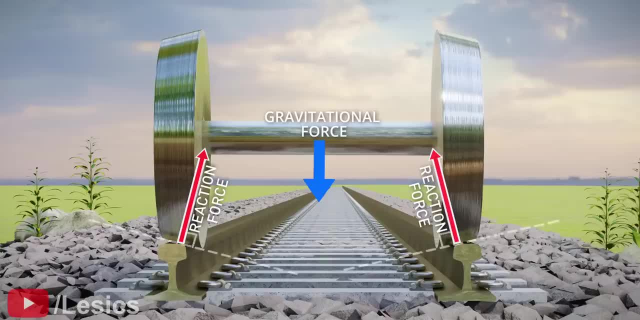 are shown here. The reaction forces will always be perpendicular to the surface of the wheel, the cone. When the wheels are centered, the horizontal components of these forces cancel each other out. Now assume that, due to some reason, the wheels have moved to the right. 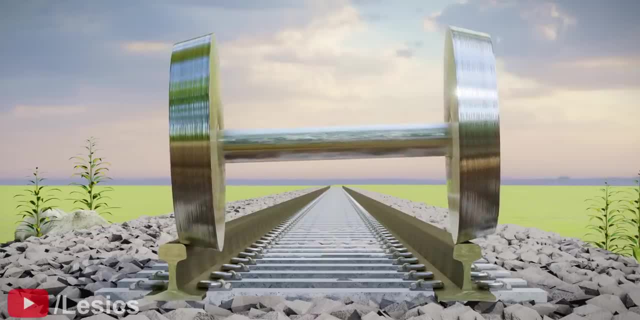 One interesting thing happens to the train's wheels when it moves along the axis. Did you notice? It is clear from the visual that the whole train wheel set tilts, as shown? Along with this tilt, the normal forces also get tilted, If you do a force analysis. 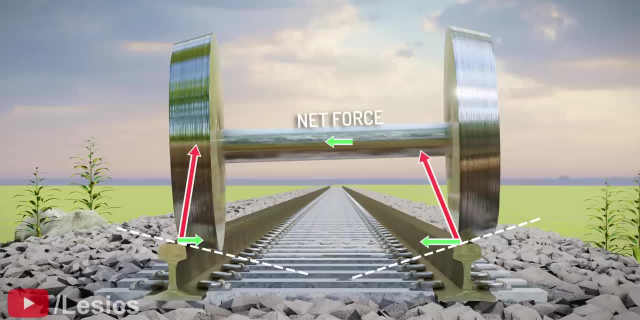 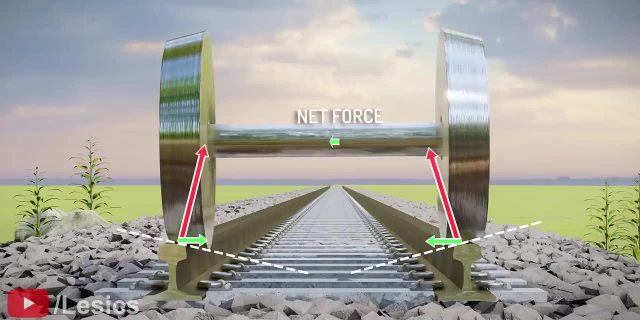 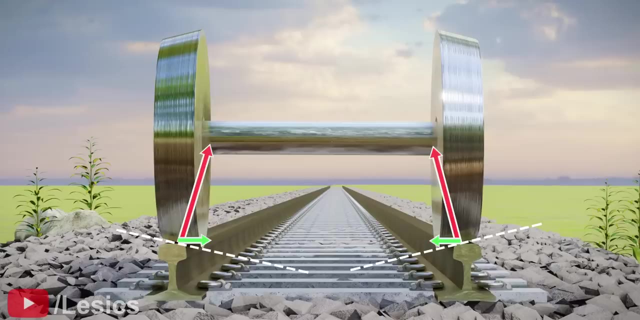 in this condition, you can see that there will be net force towards the left direction. This force will bring the wheels automatically to its center. As the wheels approach the center, the self-centering force will disappear. What a simple but brilliant technique to self-center the wheels right. Flanges are fitted on both the sides of the wheels as a result of this tilt. If you want to see how this is done, you can click on the link in the description below. If you want to see how this is done, you can click on the link in the description below. 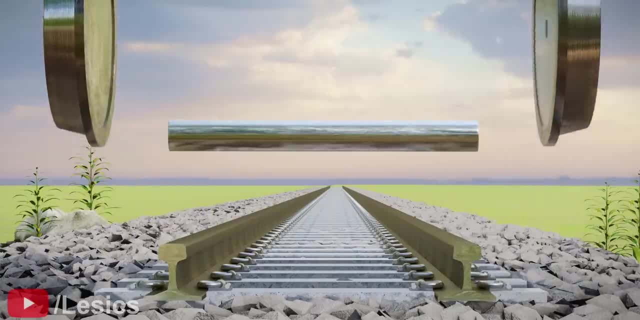 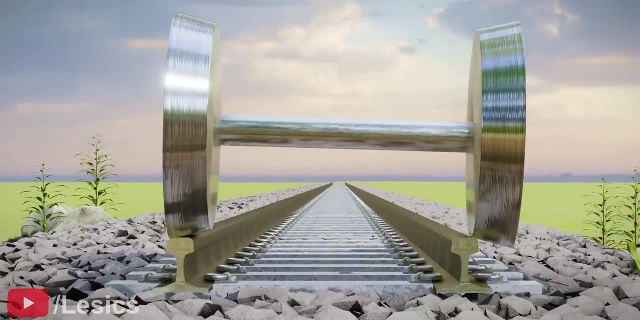 For fun, let's assume that the train's wheels are in the opposite angle Here. if you do the same force analysis during a right displacement, you can see the net force developed is again towards the right. This is why, for this wheel geometry,